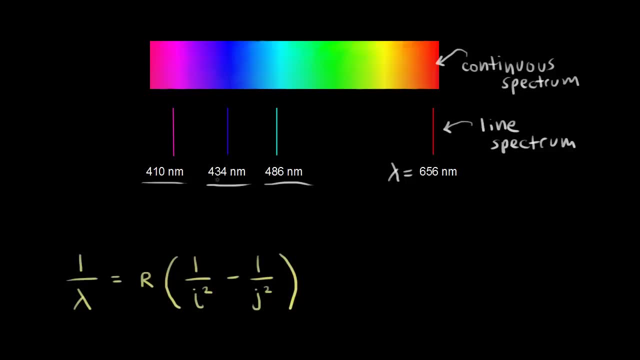 where those wavelengths come from. And we can do that by using the equation we derived in the previous video, This equation, the Balmer-Rydberg equation, And you can see that one over lambda. lambda is the wavelength of light that's emitted. 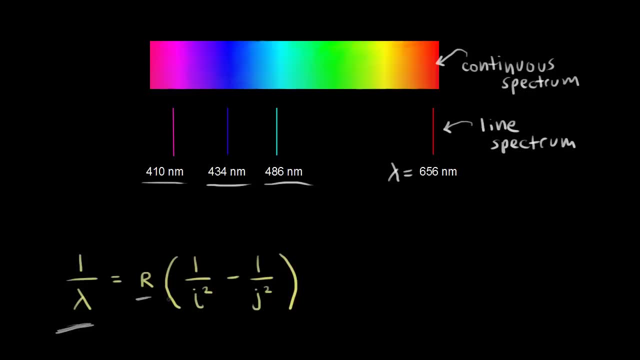 is equal to R, which is the Rydberg constant, times one over I, squared, where I is talking about the lower energy level, minus one over J. squared where J is referring to the higher energy level. For example, let's say we were considering 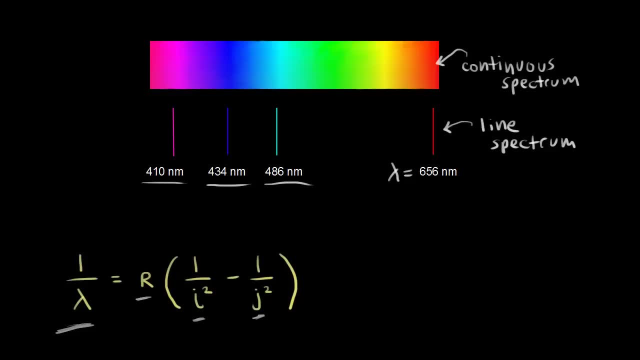 an excited electron that's falling from a higher energy level to N is equal to three. So let me write this here. so we have an electron that's falling from N is equal to three down to a lower energy level. N is equal to two. 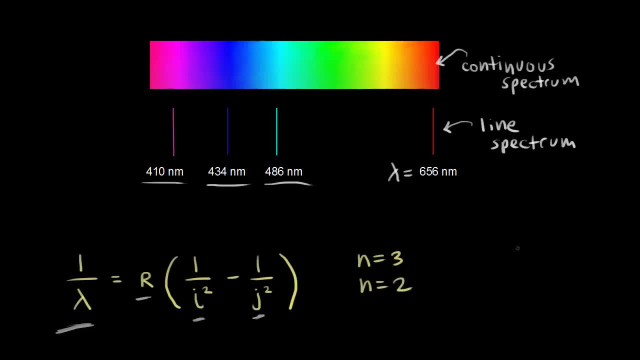 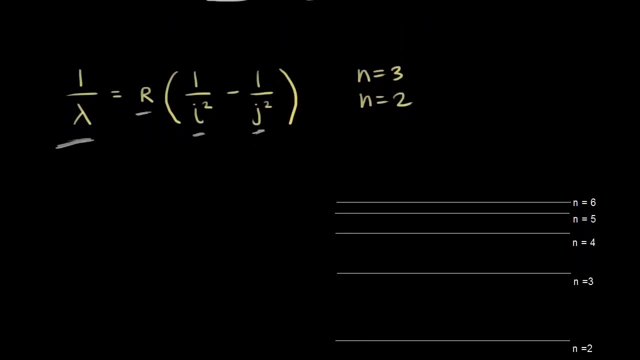 So it's going to emit light when it undergoes that transition. So let's look at a visual representation of this and then let's see if we can calculate the wavelength of light that's emitted. So if an electron is falling from, N is equal to three. 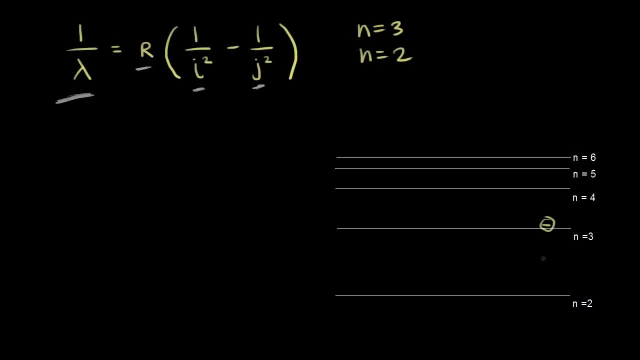 to N is equal to two. let me go ahead and draw an electron here. So an electron's falling from N is equal to three down to N is equal to two, and the difference in those two energy levels, or the difference in energy, is equal to the energy. 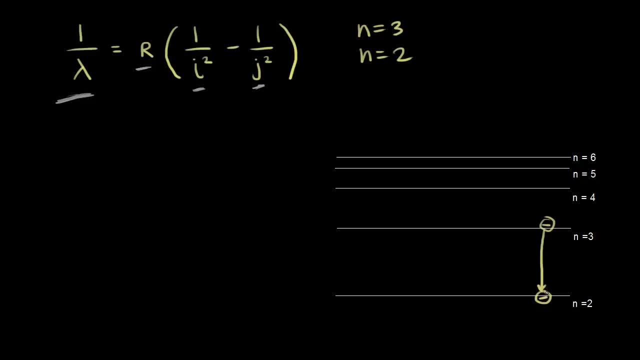 of the photon, And so that's how we calculated the Balmer-Rydberg equation in the previous video. Alright, let's go ahead and calculate the wavelength of light that's emitted when the electron falls from the third energy level to the second. 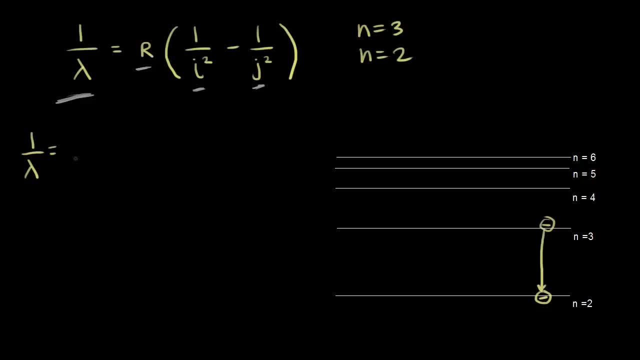 So we have one over. lambda is equal to the Rydberg constant, as we saw in the previous video, is 1.097 times 10 to the seventh. the units would be one over meter. Alright, one over I squared. 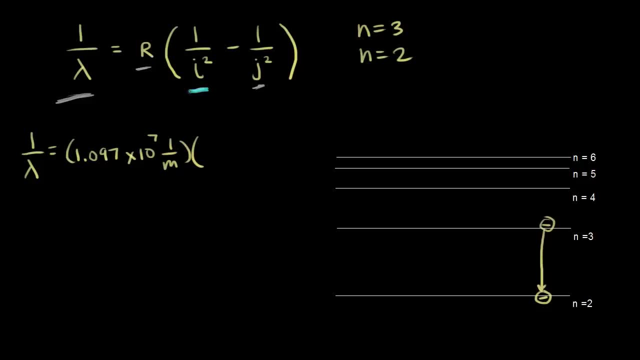 So I I refers to the lower energy level. Alright, so the lower energy level is when N is equal to two. So we plug in one over two squared And then from that we're going to subtract one over the higher energy level. 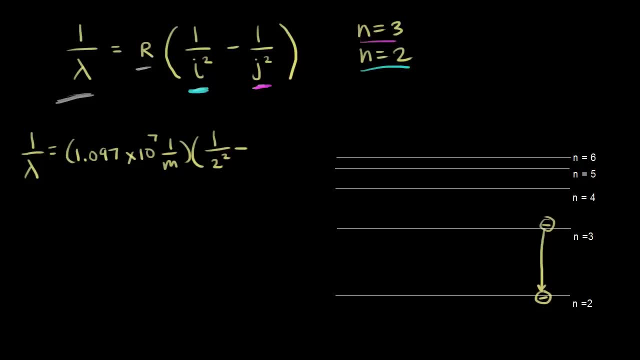 That's N is equal to three. Alright, so this would be one over three squared. So one over two squared, minus one over three squared. Let's go ahead and get out the calculator and let's do that math. So one over two squared, that's one fourth. 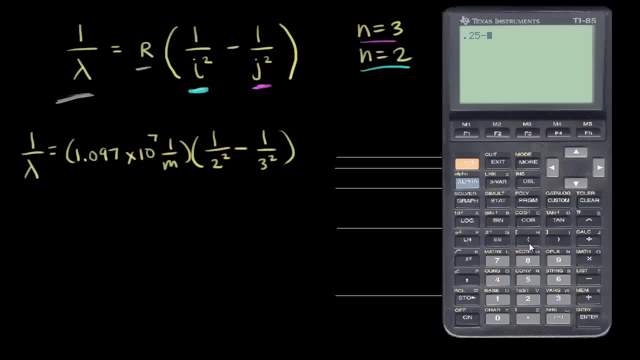 So that's .25 minus one over three squared, So that's one over nine. So one fourth minus one ninth gives us .138. repeating, And if we multiply that number by the Rydberg constant, alright, that's 1.097 times. 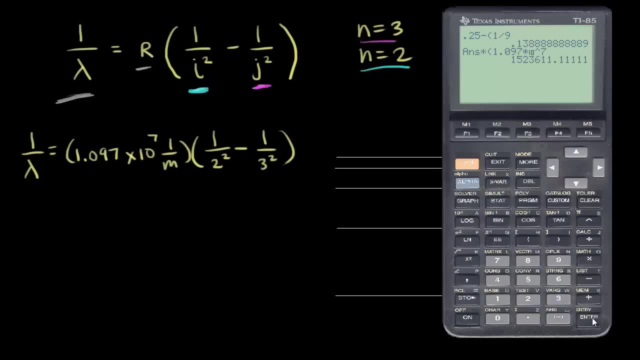 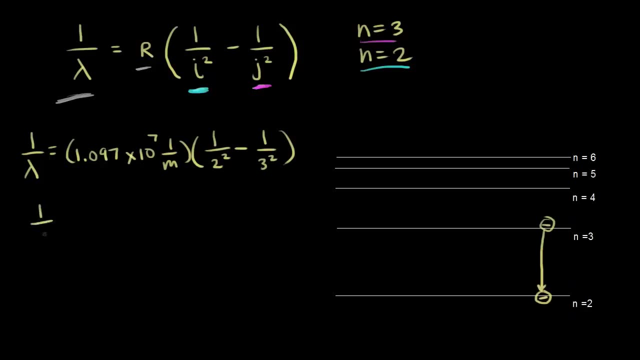 10 to the seventh, we get one, five, two, three, six, one one, So let me go ahead and write that down. So now we have one over. lambda is equal to one, five, two, three, six, one one. 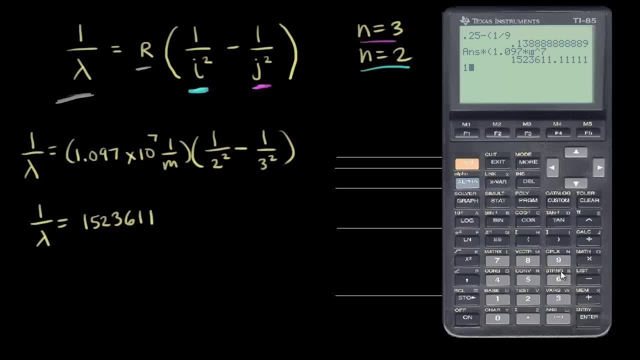 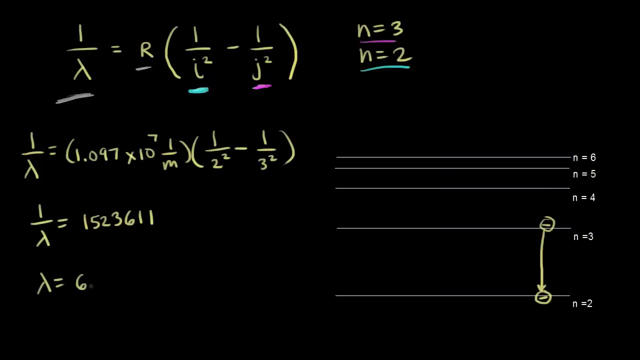 So to solve for lambda, all we need to do is take one over that number. So one over that number gives us 6.56 times 10 to the negative seven, And that would now be in meters. So we have: lambda is equal to 6.56 times 10 to the negative seventh meters. 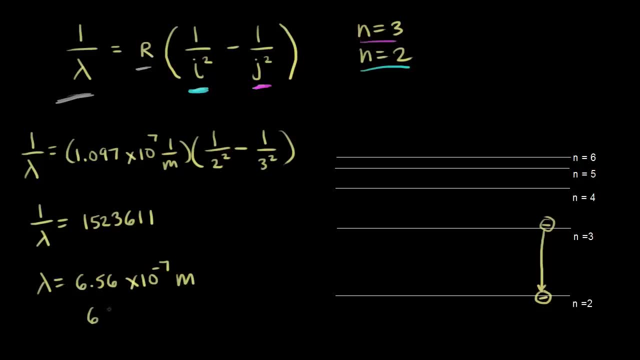 So let's convert that into: let's go like this: Let's go with 656.. That's the same thing as 656 times 10 to the negative ninth meters, And so that's 656 nanometers, 656 nanometers. 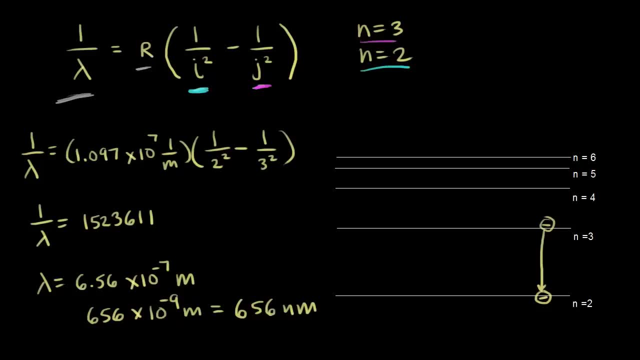 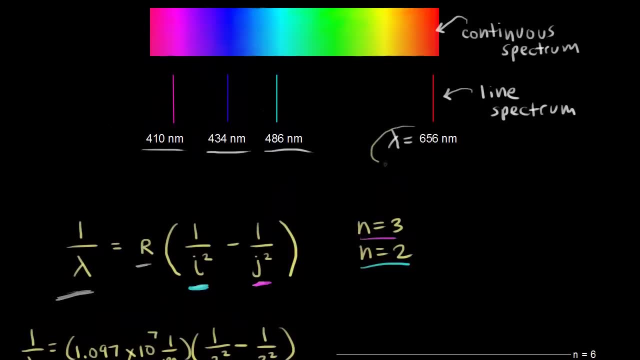 And that should sound familiar to you. Alright, so let's go back up here and see where we've seen 656 nanometers before. 656 nanometers is the wavelength of this red line right here, So that red line represents the light that's emitted. 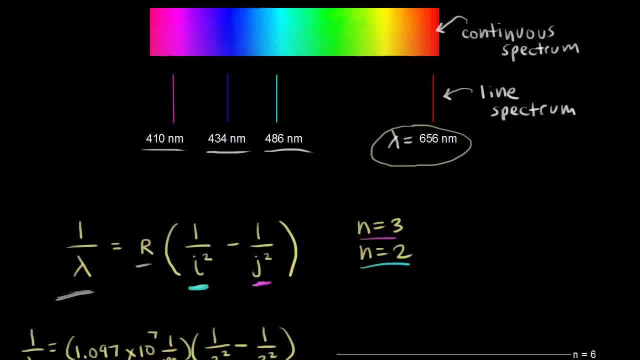 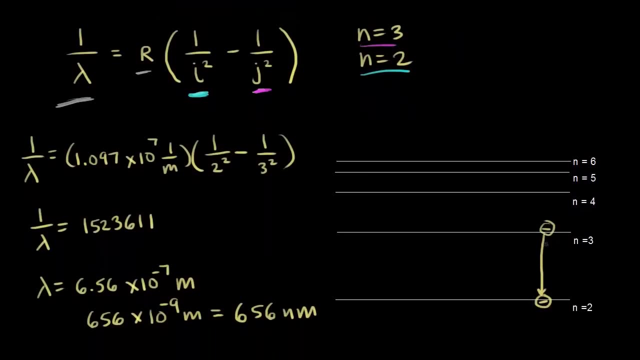 when an electron falls from the third energy level down to the second energy level. So let's go back down to here and let's go ahead and show that, So we can say that a photon right, a photon of red light is given off as the electron falls. 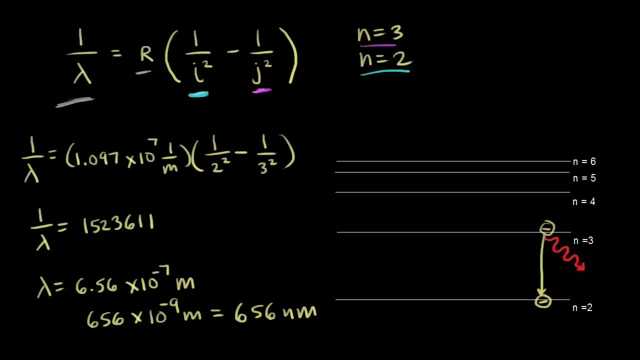 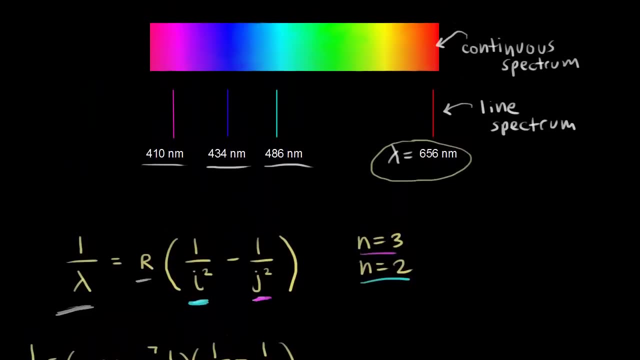 from the third energy level to the second energy level. So that explains the red line in the line spectrum of hydrogen. So how can we explain these other lines that we see, right? So we have these other lines over here, right, We have this blue-green one, this blue one. 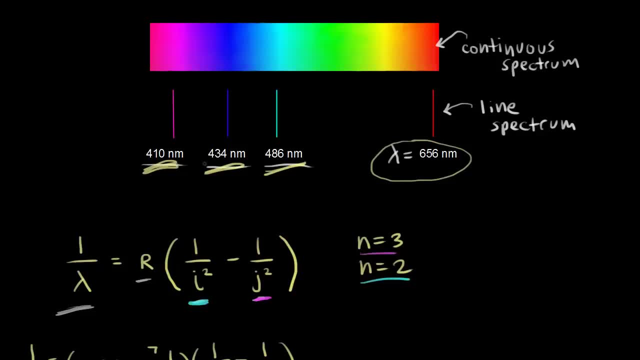 and this violet one. So if you do the math, you can use the Balmer-Rydberg equation, right, You can do this and you can plug in some more numbers and you can calculate those values. So those are electrons falling from. 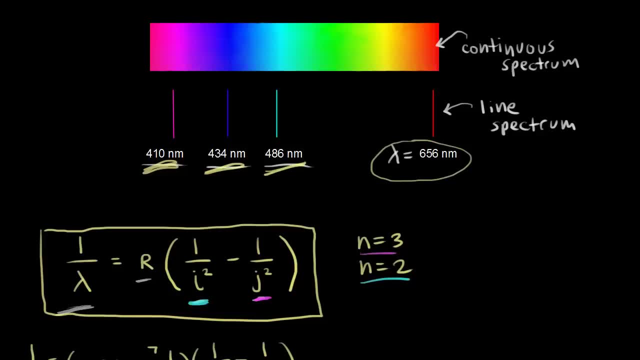 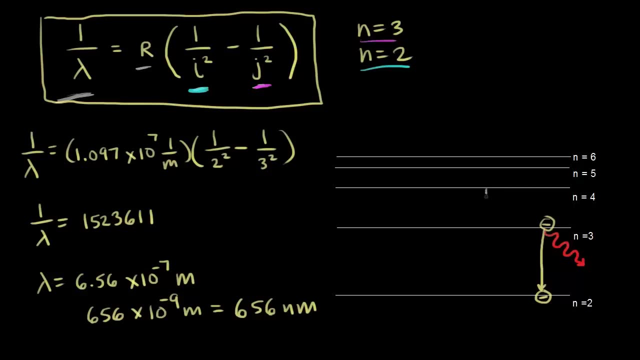 from higher energy levels down to the second energy level. So let's go ahead and draw them on our diagram here. So let's say an electron fell from the fourth energy level down to the second right. So that energy difference if you do the calculation. 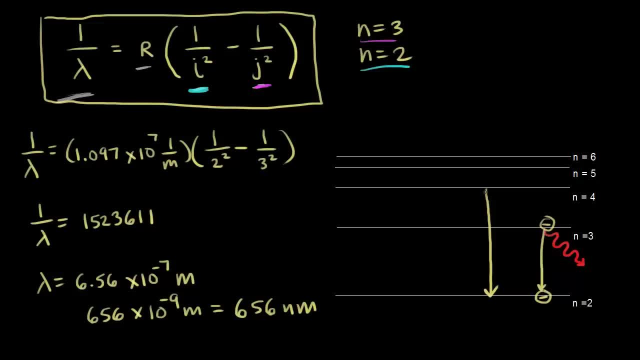 that turns out to be the blue-green line in your line spectrum. So I'll represent the light emitted like that. And if an electron fell from the fifth energy level down to the second energy level, that corresponds to the blue. So that's the blue line that you see on the line spectrum. 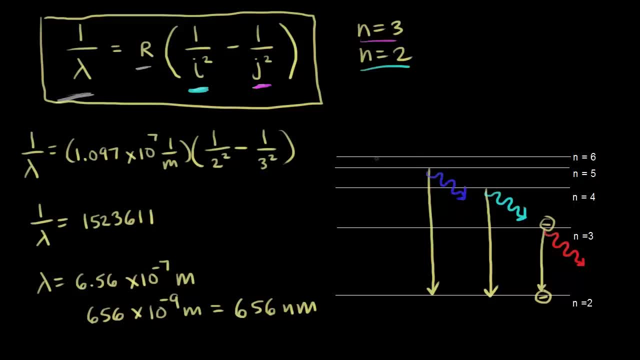 And then, finally, the violet line must be the transition from the sixth energy level down to the second. So let's go ahead and draw that in. And so now we have a way of explaining this line spectrum of hydrogen that we can observe, And since we calculated this Balmer-Rydberg equation, 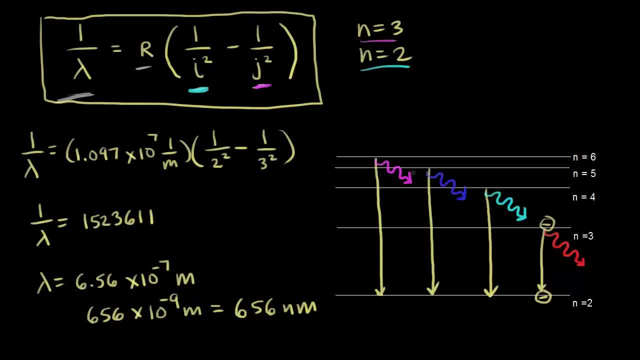 using the Bohr equation, using the Bohr model. I should say the Bohr model is what allowed us to do this. So the Bohr model explains these different energy levels that we see. So when you look at the line spectrum of hydrogen, 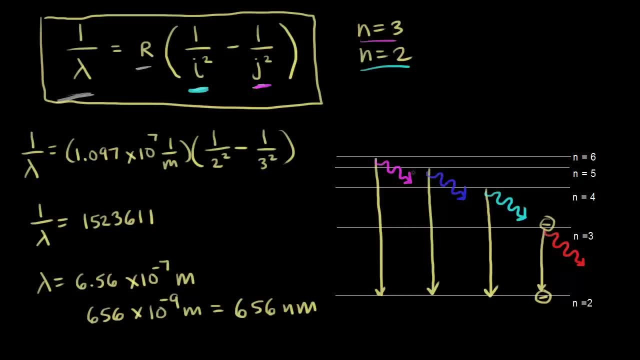 it's kind of like you're seeing energy levels- At least that's how I like to think about it, because it's the only real way you can see the difference of energy right? So energy is quantized. We call this the Balmer series. 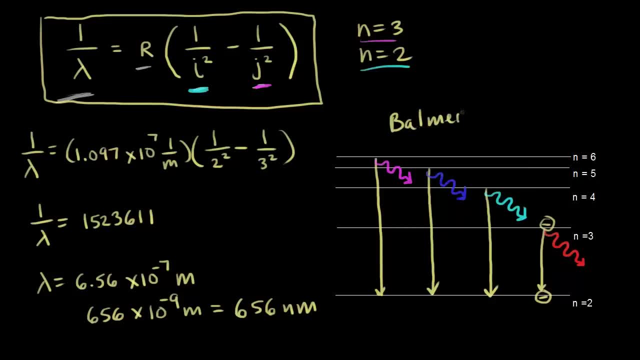 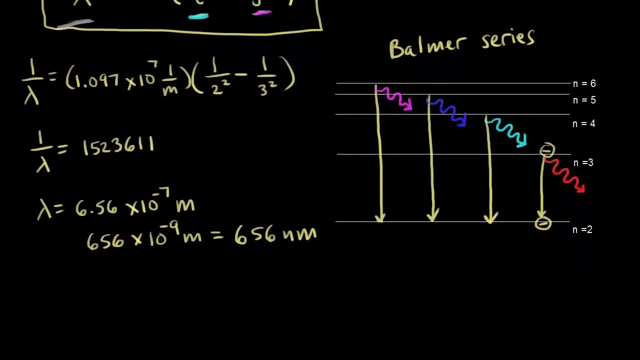 So this is called the Balmer series for hydrogen, But there are different transitions that you could do. For example, let's think about an electron going from the second energy level to the first. All right, so let's get some more room here. 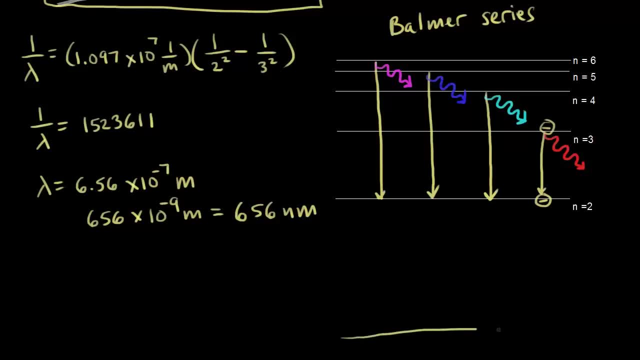 And if I drew a line in here, again, not drawn to scale, think about an electron going from the second energy level down to the first. So from n is equal to two to n is equal to one. Let's use our equation. 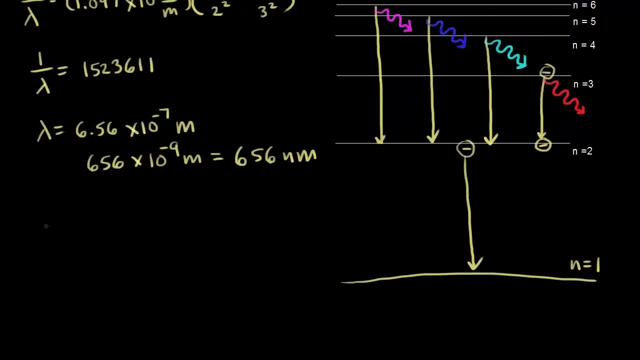 and let's calculate that wavelength next. So this would be one over lambda is equal to the Rydberg constant: 1.097 times 10 to the seventh, That's one over meters. And then we're going from the second energy level. 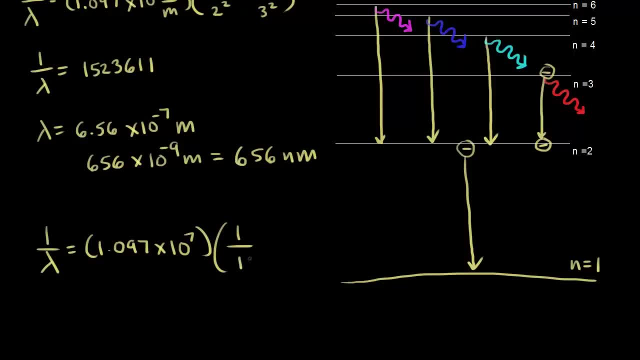 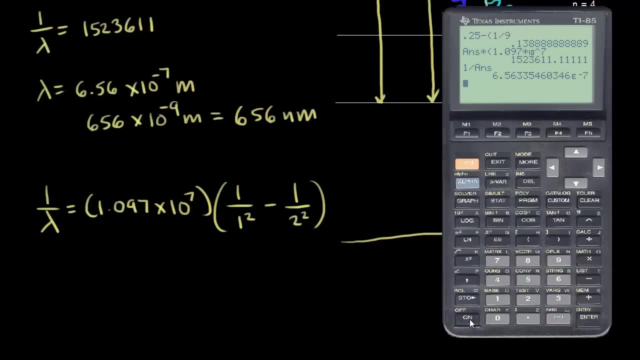 to the first. So this would be one over the lower energy level squared. So n is equal to one squared minus one over two squared. All right, so let's get some more room, get out the calculator here. So one over one squared is just one minus one. fourth, 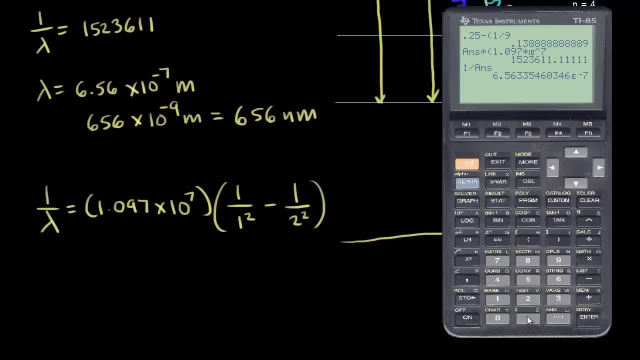 So that's .75.. So if we take .75 of the Rydberg constant, let's go ahead and do that. So 1.097 times 10 to the seventh is a Rydberg constant If we multiply that by .75,. 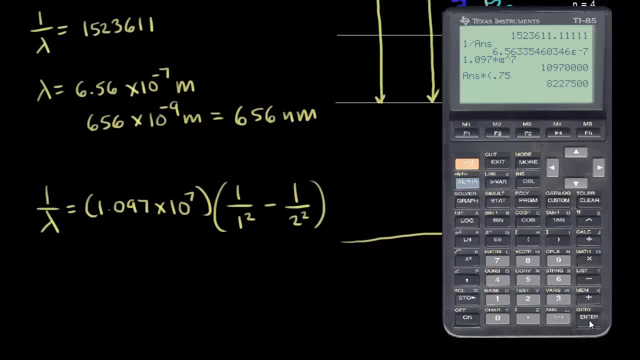 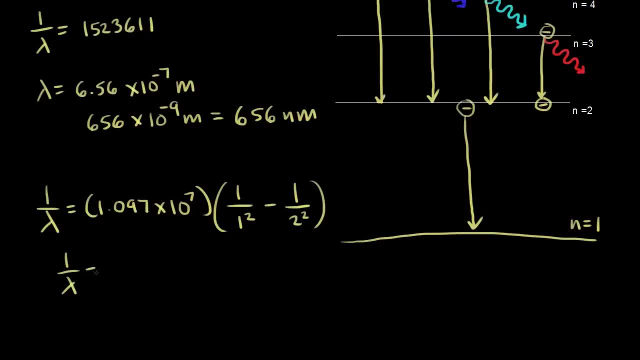 so three, fourths, then we should get that number there. So that's eight, two, two, seven, five, zero, zero. So let's write that down: One over the wavelength is equal to eight, two, two, seven. 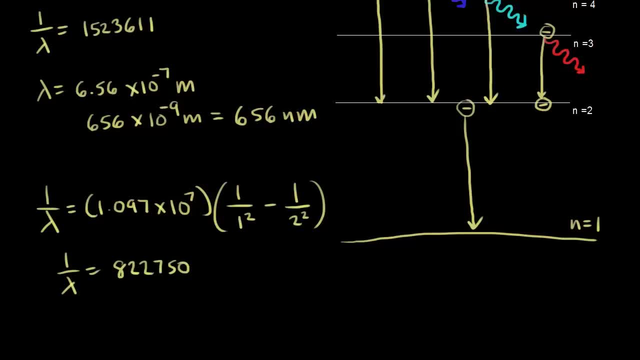 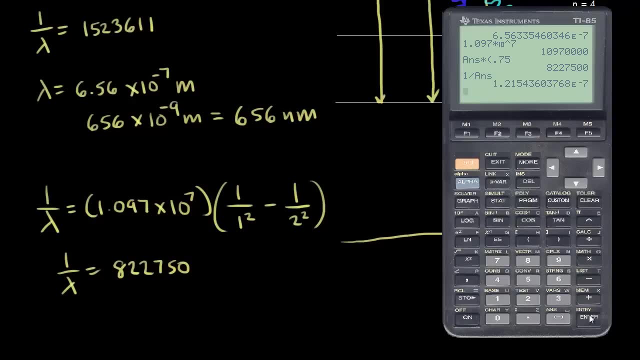 two, seven, five, zero. So to solve for that wavelength just take one divided by that number, and that gives you 1.21 times 10 to the negative seven, and that'd be in meters. So the wavelength here is equal to one point. 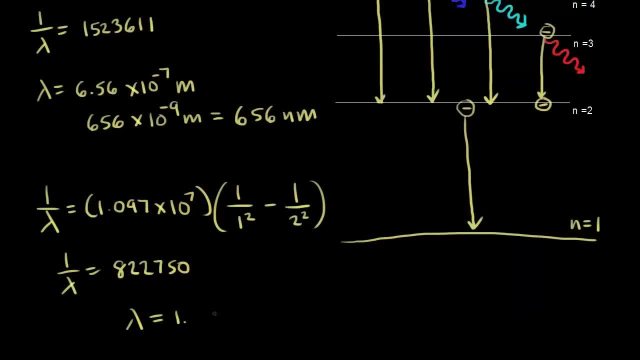 let me see what that was again: 1.215, 1.215 times 10 to the negative seventh meters, And so if you move this over two, that's 122 nanometers. So this is 122 nanometers, But this is not a wavelength that we can see. 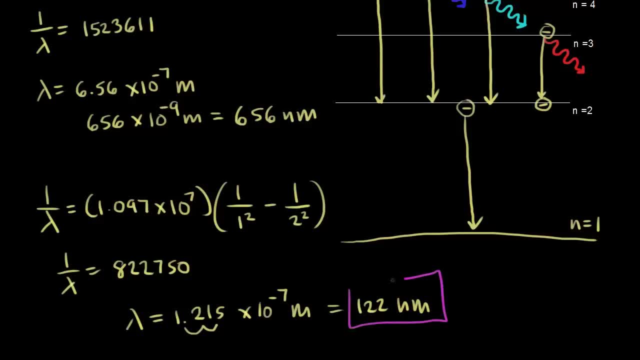 So 122 nanometers. that falls into the UV region, the ultraviolet region. So we can't see that. We can see the ones in the visible spectrum only, And so this will represent a line in a different series And you can use the Balmer-Rydberg equation. 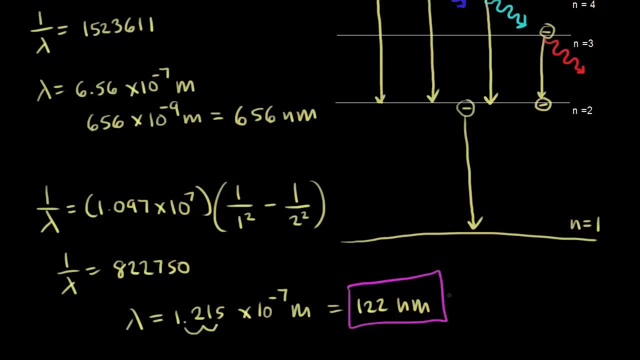 to calculate all the other possible transitions for hydrogen, and that's beyond the scope of this video. So here I just wanted to show you that the emission spectrum of hydrogen can be explained using the Balmer-Rydberg equation, which we derived using the Bohr model of the hydrogen atom. 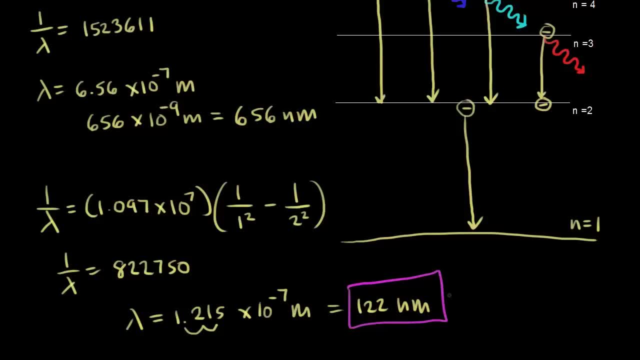 So, even though the Bohr model of the hydrogen atom is not reality, it does allow us to figure some things out and to realize that energy is quantized.